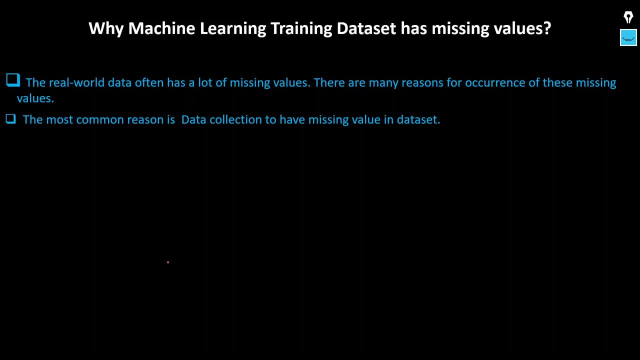 Hello everyone. today we are going to discuss about the missing value. In this today video, we will discuss what is the missing value, what would happen if we will not impute the missing value in the real-world data set while training our machine learning model, and we will see what. 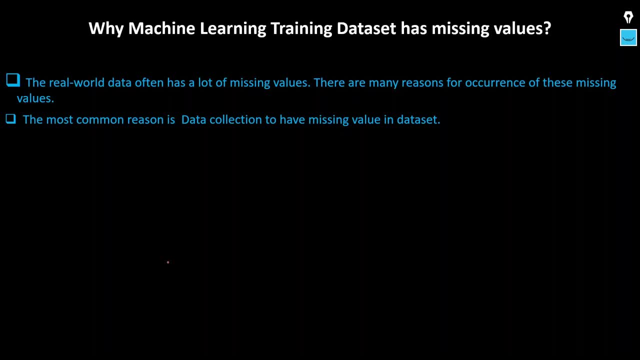 are the different techniques we use to perform to impute the missing value in the real-world data set. So let's start Why machine learning data set has a missing value. What we will do, we will check. the real-world data often has a lot of missing value and there are many reasons. 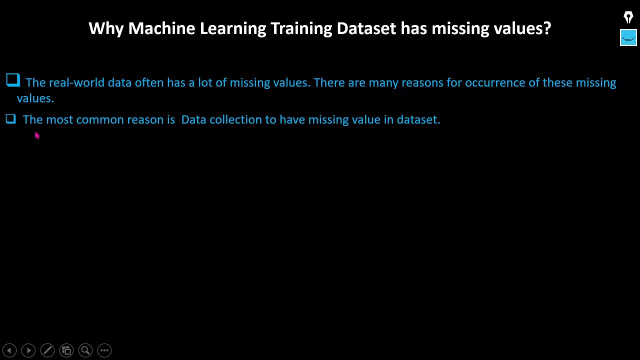 for occurrence of this missing value. So what are those reasons? The main reason is data collection. So main reason is data collection. Let's, we are collecting the data from different sources. So when we collect the data, so what happened some time? let, these are the different-different data sources. So once we 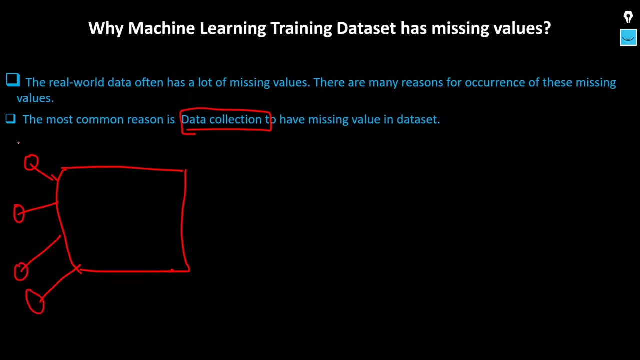 collect the data. so what happened? let's say I am collecting the employee information from region UK, Asia and US and Australia. So what happened? The employees which exist here have an employee number and corresponding email Id, But the Asia region employee. 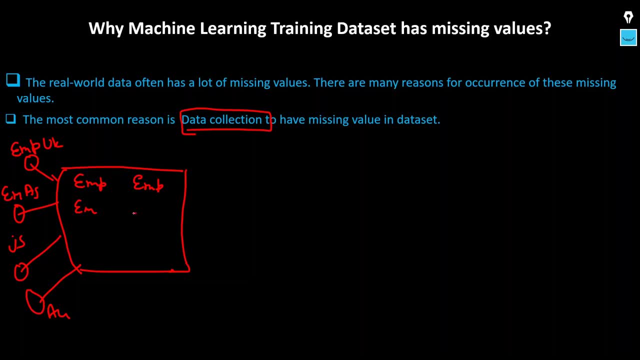 some employees doesn't mention the email Id. So that's why we will get some null value corresponding to this particular row under the employee email column. So that's why we get the null value or the missing value in this particular table. employee table in the column. 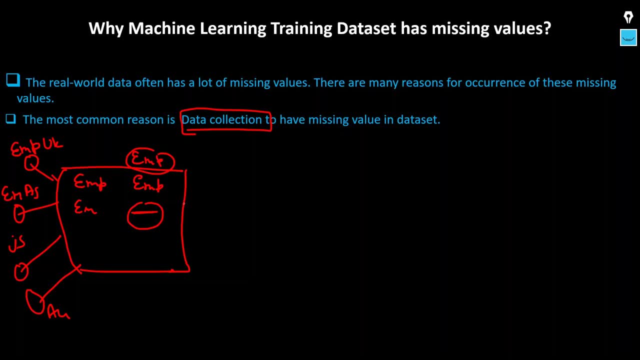 employee. So this is the reason: if you will work in the real world data set, you will get many missing values, which we used to have in many columns. Another very good example is that once you provide the feedback, once you provide the feedback, there are many like there are many. 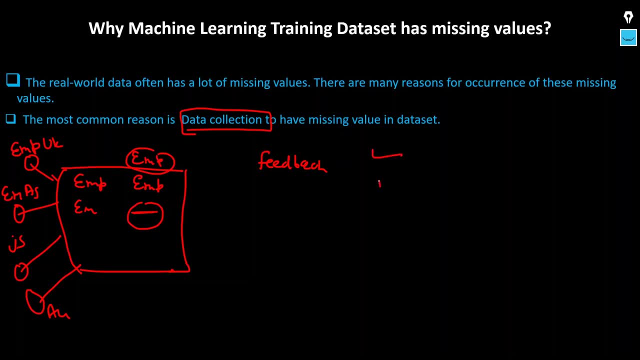 checklists where you will have to check like first point, second point, third point, fourth point, and in last command they mention the others. So what we used to do in the others section, we don't provide too much information. Somebody leave blank this particular other section, somebody only mention. 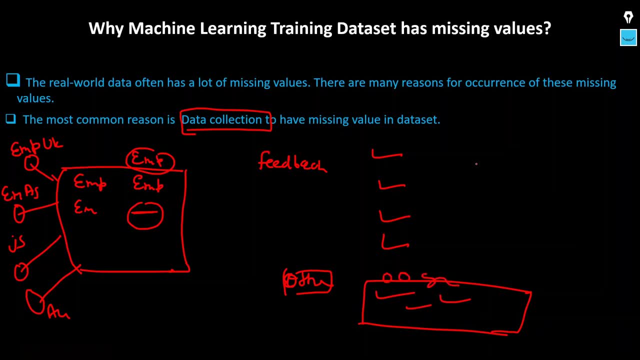 good old. somebody doesn't mention anything. so that's why whenever we like feed this data in any like in any database. so what we used to get, we get others column many null values because many customer doesn't mention any feedback in the others section. so that's why we used to get many nulls value in the other column. 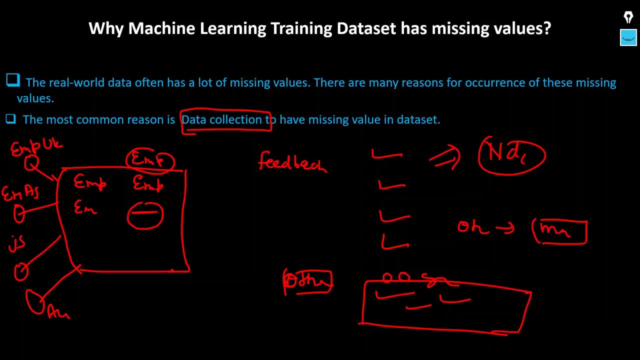 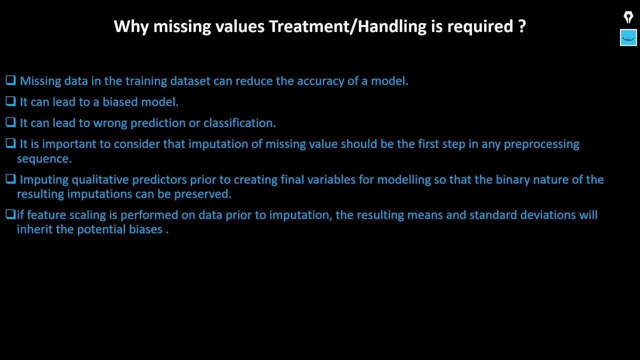 this is the main reason we get missing value in most of the columns in the real world data set. so let's start the next detail: why missing value treatment and handling is required? because we have the null value in the data set. so what would happen? what would happen if we will not treat or handle this missing value? first, 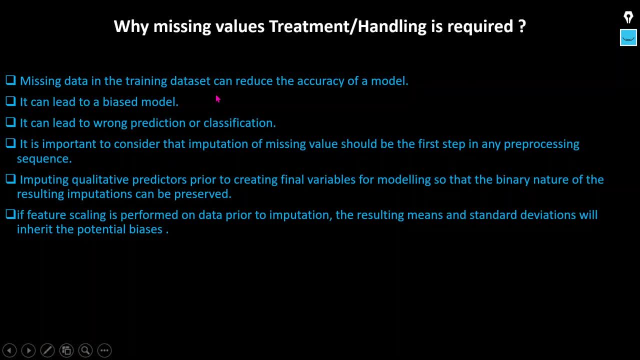 one is that missing data in the training data set can reduce the accuracy of the model. if we select some columns for our machine learning, model training, and if there are null values, if there are null values in some columns, so what would happen? it will reduce the accuracy of the model. it will reduce the accuracy of the model. so we try to fill. 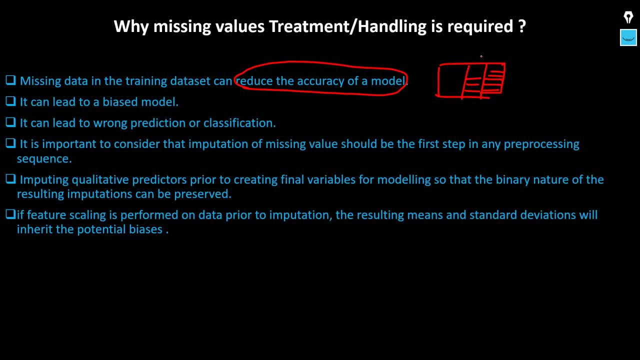 these null value or impute these null values in some column wherever we have the missing data. second one: it can lead to the biased model. it means that the data set can reduce the accuracy of the model if we select some columns. so this will lead to the bad prediction in the null value. 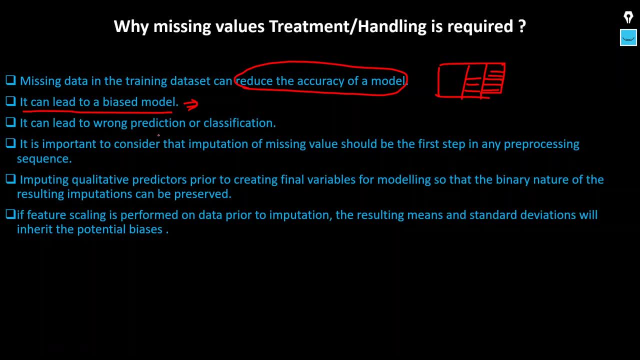 training. so this means that I will explain anyway. next slide, then you will get some more details. it can lead to wrong prediction or classification, so this will you will also get in our next slide by one example. it is important to consider that imputation of the missing value should be the first step in any 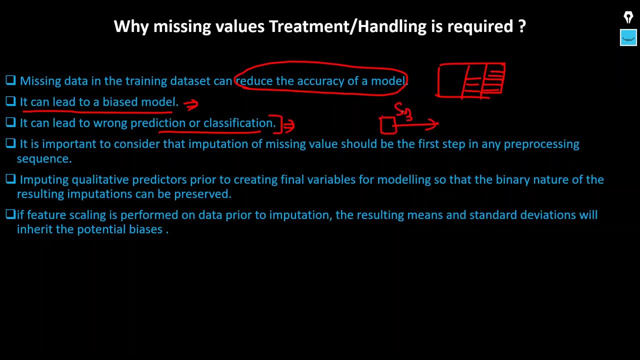 pre-processing sequence. it means whenever we collect the data from our data lake machine learning model for our machine learning model, so after that we do the data cleaning. so in the data cleaning, first B, so what we used to perform first B, try to do impute the missing value. try to impute the missing value. it means we 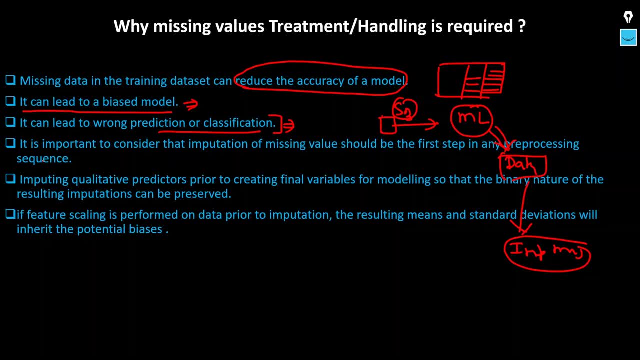 have to first impute the missing value and imputing qualitative predictors. it means imputing categorical predictors prior to creating final variable for modeling, so that binary nature of the resulting imputation can be preserved. it means let's. this is our gender column. this is our gender column where we 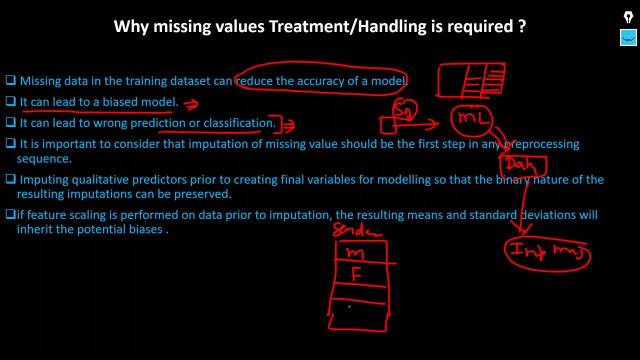 mention male, female, let, there are hundred rows, so out of hundred rows, 20 rows data is missing. so without imputing these data, if we do encoding on this data, so what would happen? we will not able to preserve the. we will not able to preserve the. 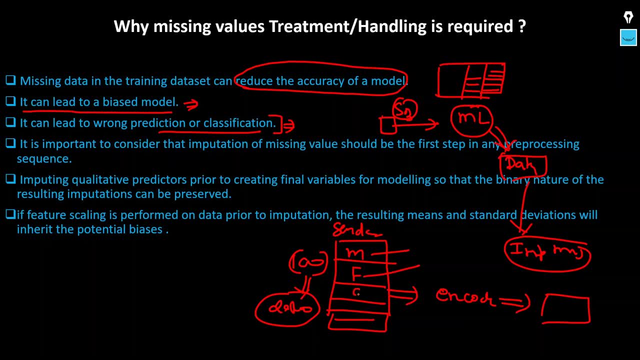 actuality meaning of the gender. because wherever we null, we will not able to get anything. so that's why it is always recommended to first impute the categorical variable missing value, then after that do the encoding encoding means: categorical variable missing value, and then after that do the encoding encoding means. 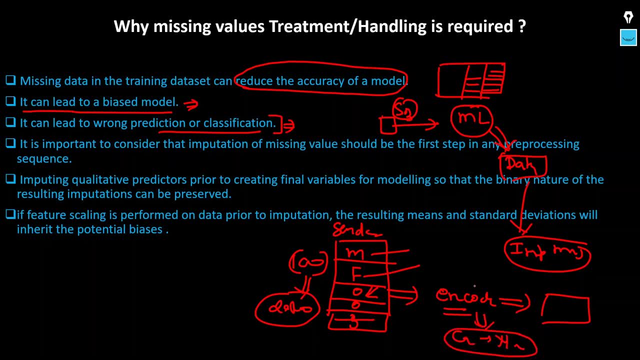 convert categorical to numerical. so this encoding I will cover during the feature engineering. if feature scaling is performed on the data prior to imputation, the resulting mean and standard deviation will inherit the potential bias. so what does it mean? like: this is your numerical variable temperature. this is 30, this is 40, this is 45. there are some values we have. 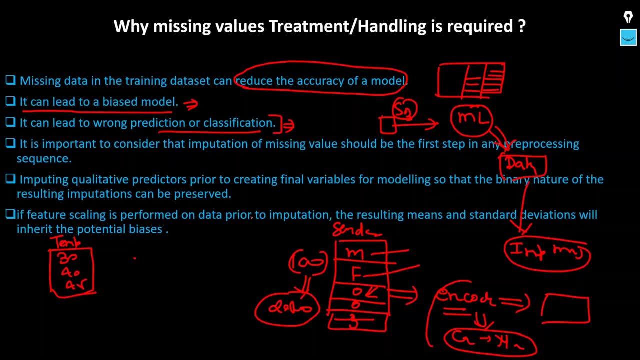 inside the temperature column. so what it is saying: a given day is noise level, so this is the value that we have inside the S column. so what it is saying, if we will do the feature scaling before the imputation, let. this is your temperature column and there are 100 rows out of 100. there are 20 rows data. 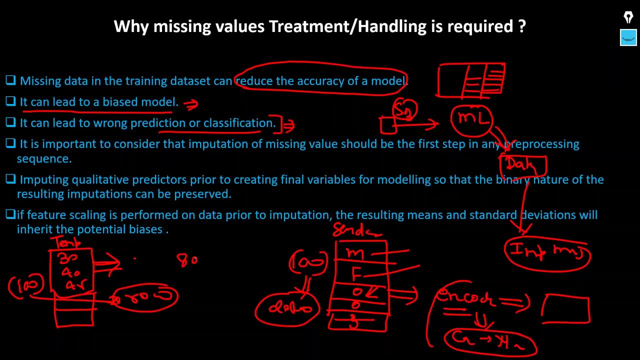 is missing. it means out of 100, we have only 80 rows where we have the temperature data. so if we will do the feature scaling, feature scaling means make the data in the same range, like 0 or 1, so there are many methods that we 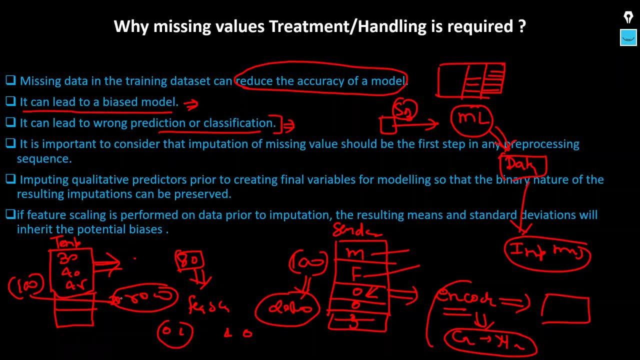 will also cover in the feature engineering. so just understand that in the future is scaling be try to make the data in a same range, either 0 or 1 or 0, and standard deviation is 1, so doing that if we will perform feature engineering before the missing value, in that case what would happen? we will 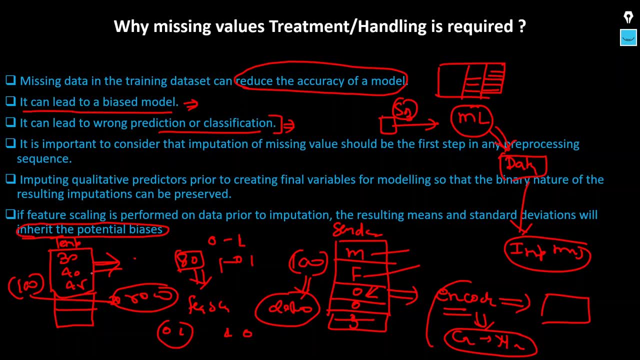 inherit the potential biasness, it means bias our model, So that's why we perform the missing value imputation prior to feature scaling. So let's understand these two topics: why it can lead to the biasedness in the model and why it can lead to wrong prediction and classification. by one example here: 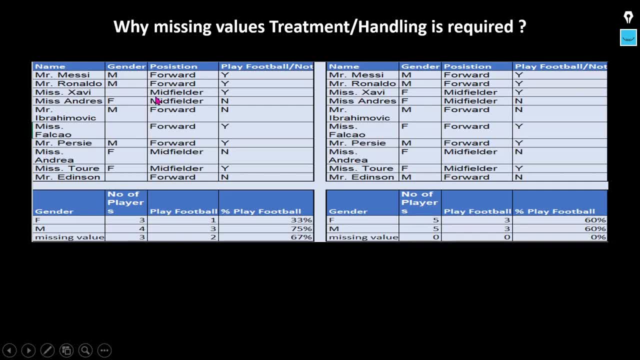 So this is the player's data- who play the football or who doesn't play the football- and we segregate the data with the help of female and male. So here we can see that. so we can say: female is three who play the football. total we can. 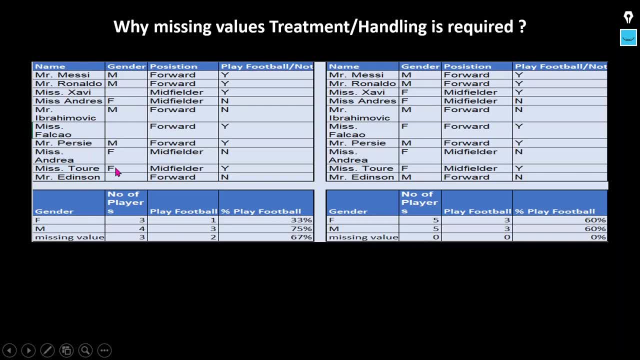 check how many females we have: one, two, three and, out of three, how many females who play the football. No, then female. no, female is, yes, only one. we have only one female who play the football, and here we can see that, out of four male candidate, there are only three males who 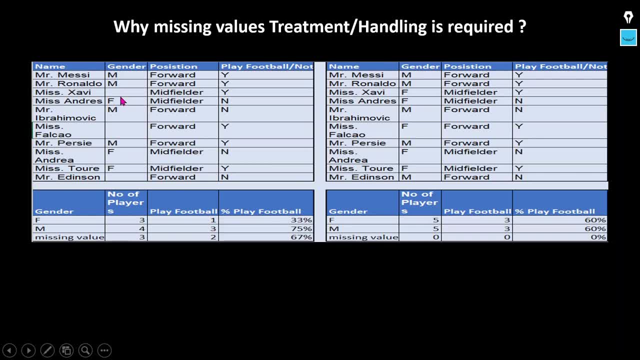 play the football And how many missing value. we have one, two, three. we have three missing value. So, out of three, how many candidates who play the football? out of three, two candidates who play the football. So in this way, if we will get a percentage player, football. 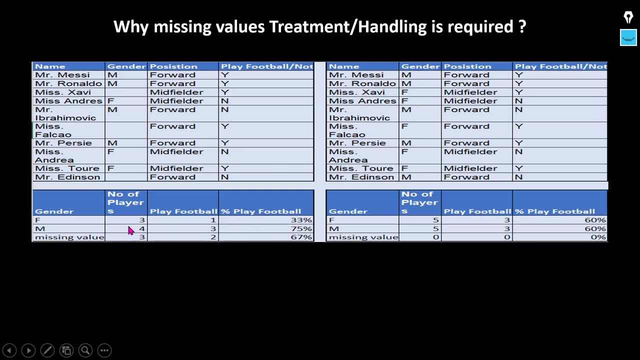 So here we can say that 33% candidates of the female who play the football and in male candidate, So 3 out of 4, it means 75% male candidate play the football. and missing we have 67. So what we did? we impute this missing value. 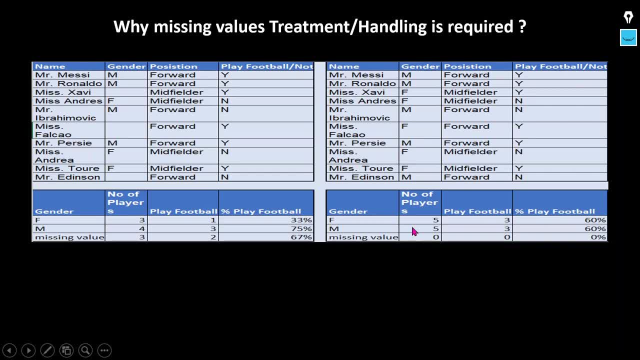 Then after that we are gonna check the analysis Here. number of players: female is five and also male is five. Number of play football: three and male is also play the three. So we can check what is the percentage of the female candidates who play the football. 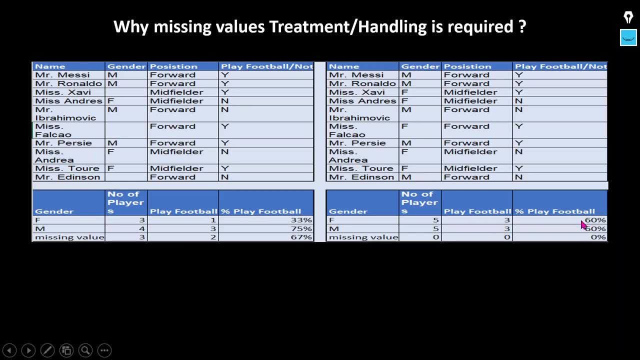 three out of five who play the football. So that's it. So we can say that 60% female candidate play the football and 60% male candidate who play the football Earlier. we are getting the 75. now it is get reduced to 60.. 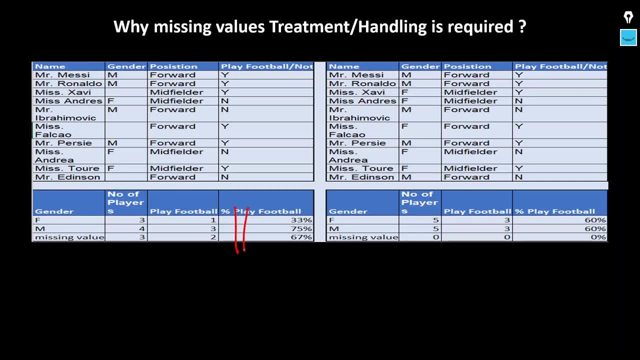 So we can clearly say that if we will use this data set to train our machine learning model, in that case it will be more biased to male candidate. It will be more biased to male candidate. And here, if we will use this data set to train our machine learning model, in that case we 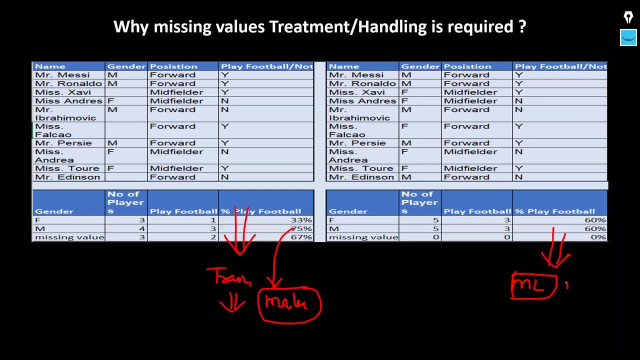 can say that it will not be biased between male or female. So we can say that if we will not impute the missing value, it can lead to the biasness And it will also not provide the good prediction or classification. And if we will use this, then we will be able to classify properly. 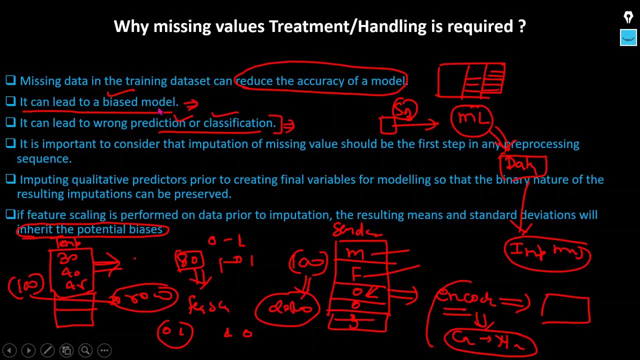 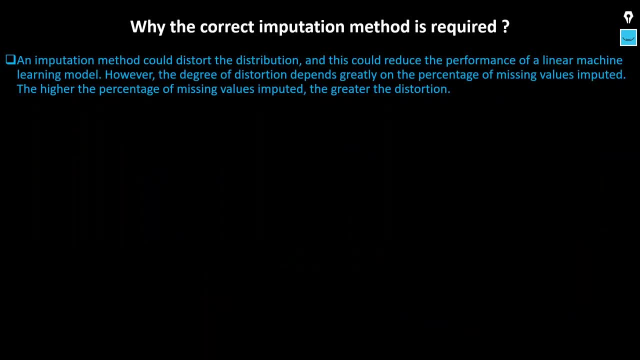 So that's why I mentioned that it can lead to biased model If we will not impute, And it can lead to the wrong prediction and classification. Why the correct imputation method is required. It means let's we know we have the missing value in this data set. 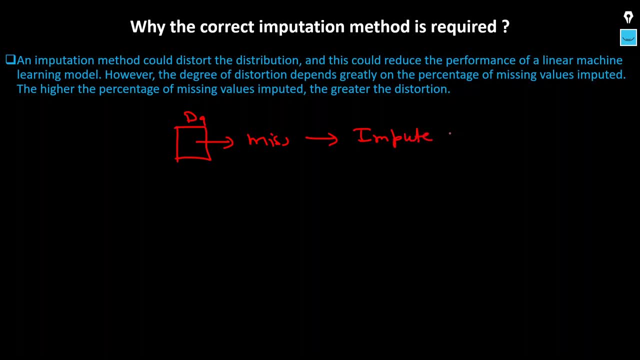 So now we have to impute the missing value, And we know many methods by which we can impute the missing value. What? why the correct imputation method is required. Let's, we know 10 methods, So we have to select the correct imputation method. 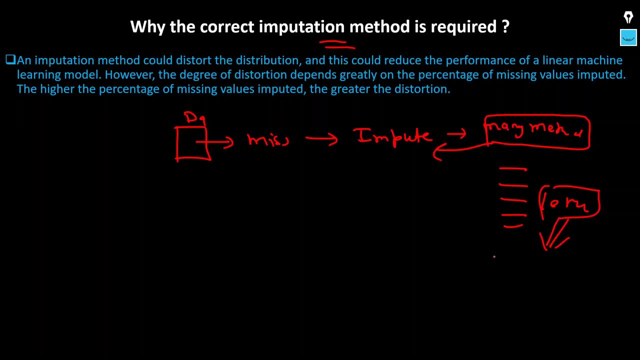 So we have to select the correct imputation method. So we have to select the correct methods. Why, using that, we can impute the correct missing value in that particular data set. Let, this is our data set. In our data set, these are the fair. there are 100 rows out of 100 rows. 50 rows data is missing. 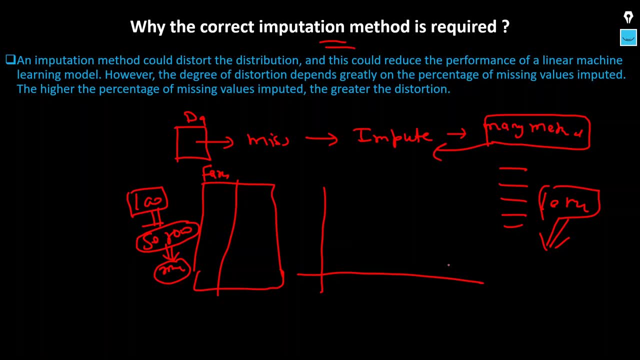 And if we will use the mean value, in that case, let's in initially distribution. is that? initial distribution is that this is your left skewed. Might be our model will work like that, Or might be our model will work like that. So what would happen if the distribution is not same? 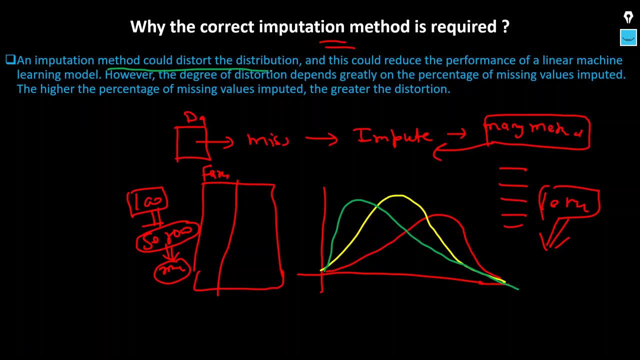 As you can see, that an imputation method could disturb the distribution. It is mentioned that if we will not use imputation method, in that case our distribution may get impacted of the original data sets And this could reduce the performance of the linear machine learning model. 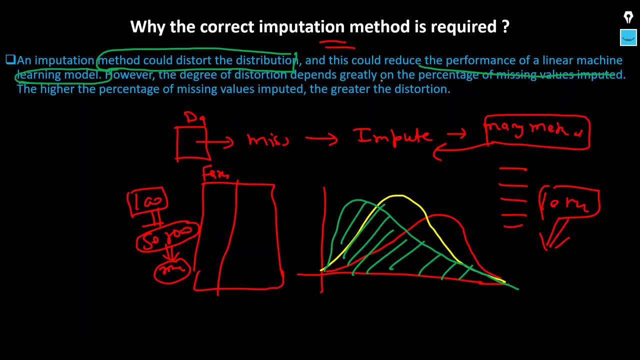 How to use linear machine learning model. However, the degree of distortion depends greatly on the percentage of the missing value. Because we have 50% might be get impacted too much, But if we have a very little amount of like, we can see that 20 or 10% then it will not. 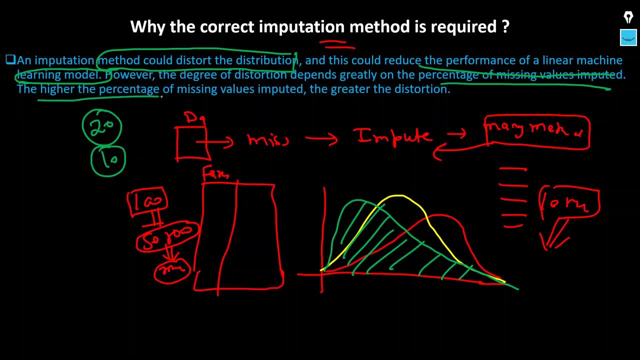 be too much impacted. The higher the percentage of the missing value imputed, greater the distortion. As I told you, we have more missing value, then it will be more distorted. So that's why we have to select a proper imputation method. So that's why we have to select a proper imputation method. 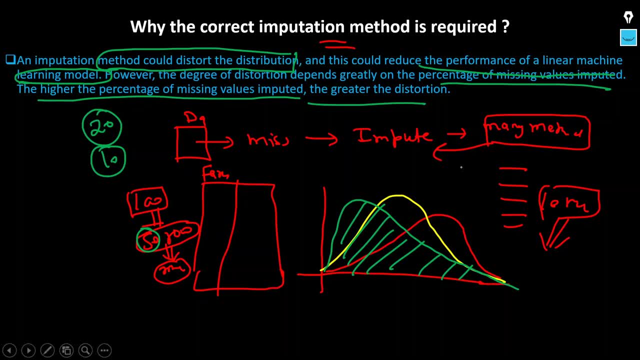 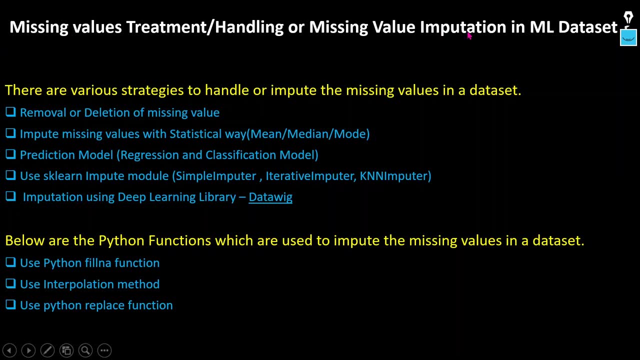 So that's why we have to select a proper imputation method to impute our missing value. Now let's discuss missing value treatment or handling the missing value, missing value imputation- There are many names. we call it handling the missing value, imputation of the missing value. 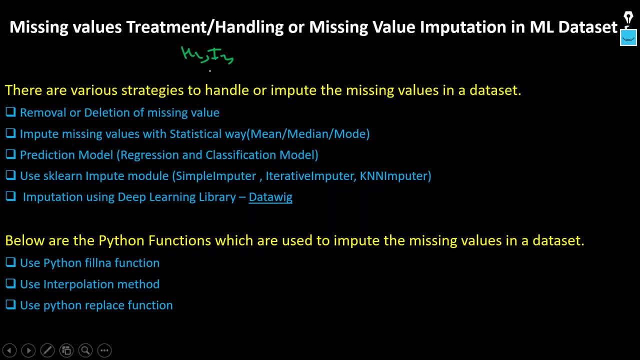 or treatment of the missing value All are same. There are various strategies to handle or impute the missing value in the data set: Removal or deletion of the missing value. I am just describing what are the methods we use to perform during our data cleaning. 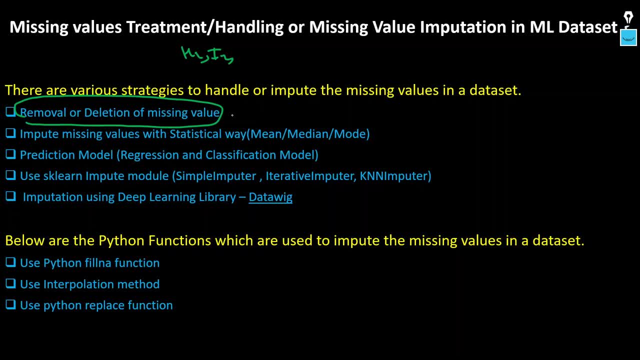 to impute the missing value. In our next video I will explain all these method by using the hands on. So removal or deletion of the missing value. Impute missing value with statistical way. It means we can use the mean of that particular column or median, or the mode of that particular. 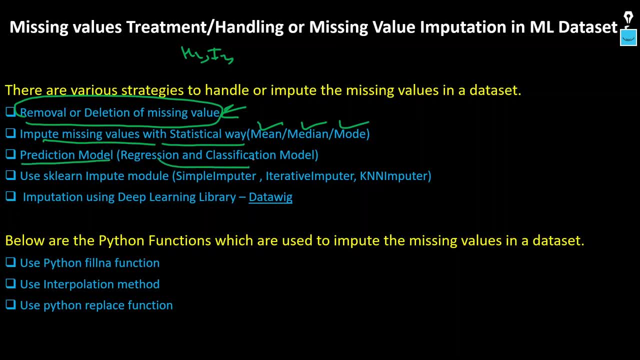 column And the prediction model. We can use the regression and some other classification model And the prediction model. We can use the regression and some other classification model to predict the missing value. We can use scikit-learn impute model like simple imputer, iterative imputer or a canon. 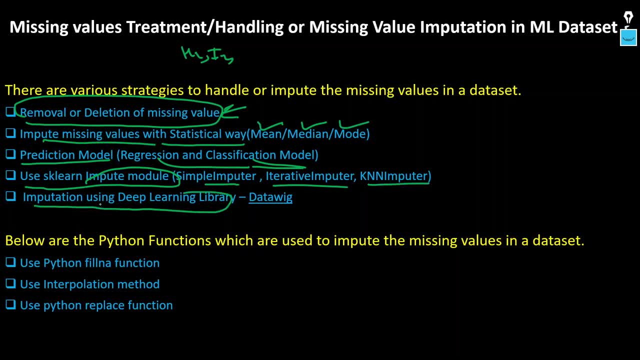 imputer to impute the missing value. Imputation using deep learning library database. So we can also use this library to impute the missing value. Below are the python functions which are used to impute the missing value in the data set. There are some python functions: